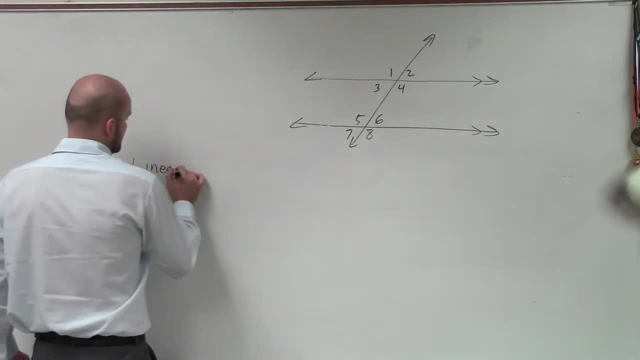 is a linear. pair is two adjacent angles. that means they share the same vertex and the same side, that make up a straight line, that have opposite rays. So I just need to figure out what two angles make up a straight line. Well guys, there's a lot of linear. 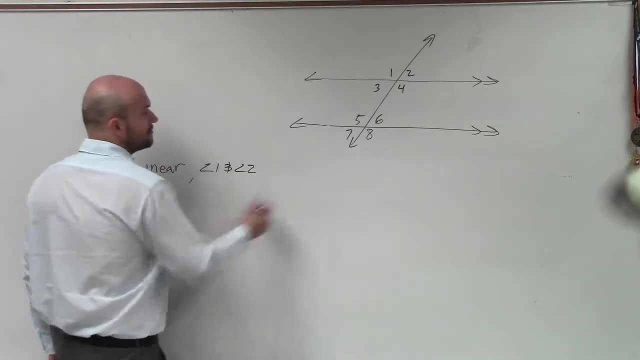 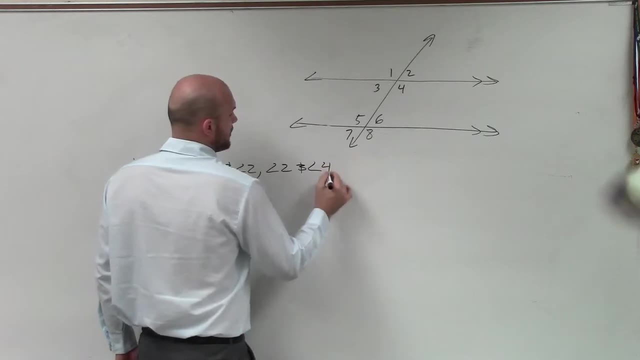 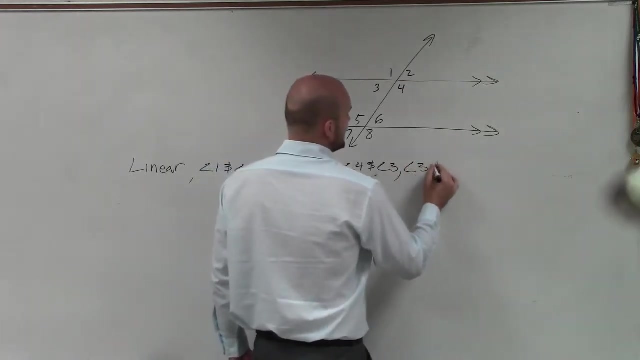 pairs: Angle one and angle two, right, Those two lines, those two angles make up a linear pair. You could say: angle two and angle four, Angle four and angle three, Angle three and angle one. Do you guys see how each one of those all make up a line? So those are all a linear. 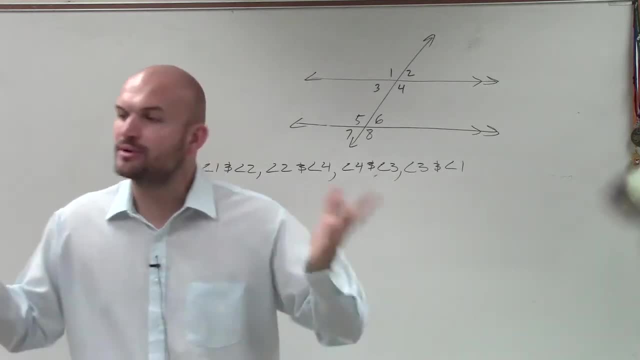 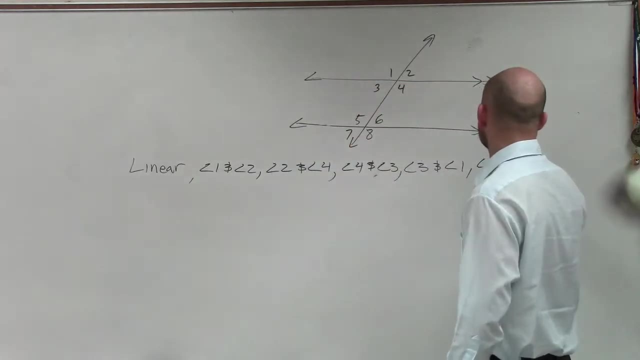 pair. And remember, linear pairs, since they make up a straight line, are what we call supplementary. They add up to 180.. Then, to continue, we could also say angle five and angle six. We could say angle six and angle eight. We could say angle eight and angle. 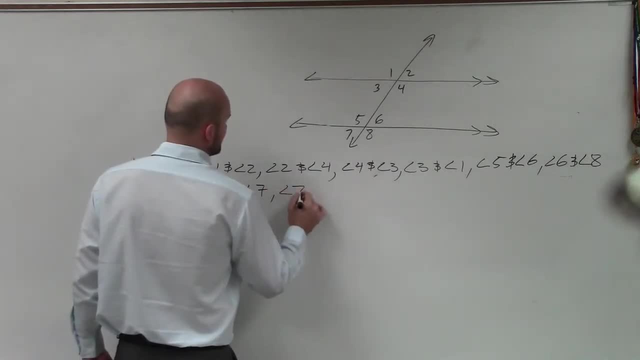 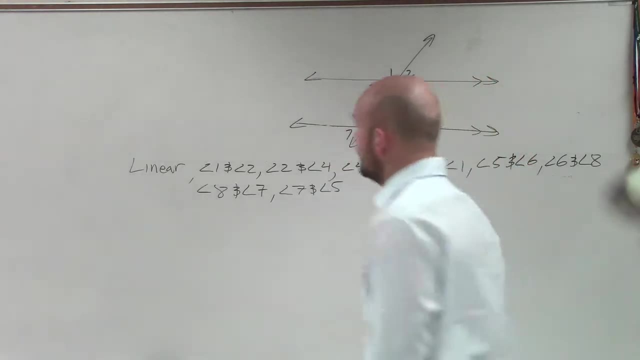 seven, And you could say angle seven and angle five. Okay, So there's a lot of linear pairs. Should have taken you a long time. The next one is vertical angles. Again, vertical angles, guys are angles. Oh, that's a linear. 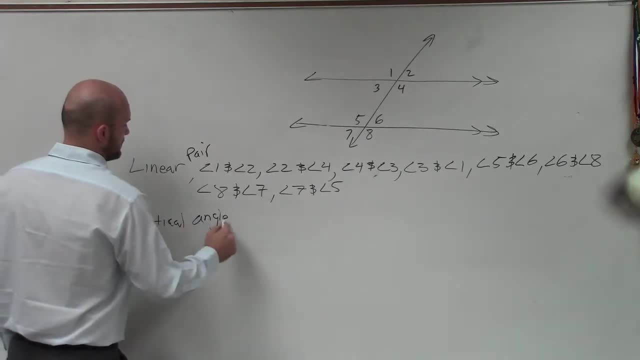 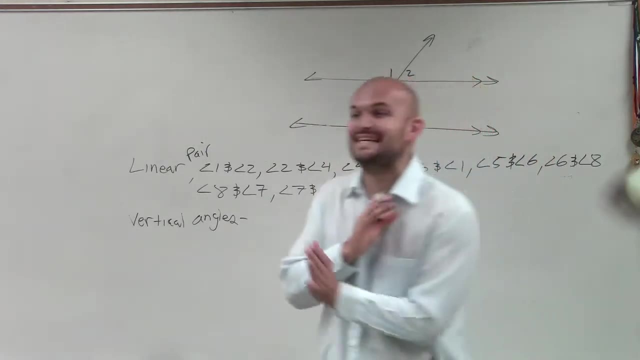 pair: Vertical angles. Yeah, So vertical angles, ladies and gentlemen, are angles, remember, that are directly across from each other on the intersection of two lines. They do not prove parallel lines, Just like a linear pair doesn't prove parallel lines. 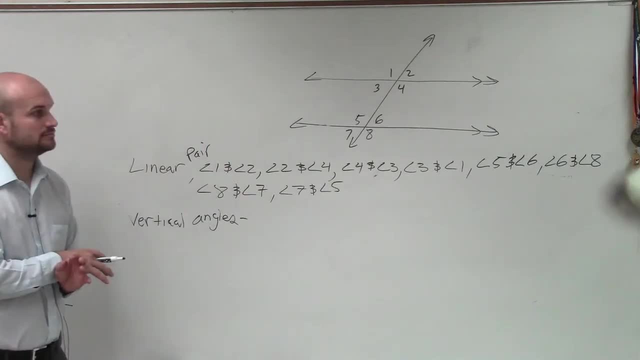 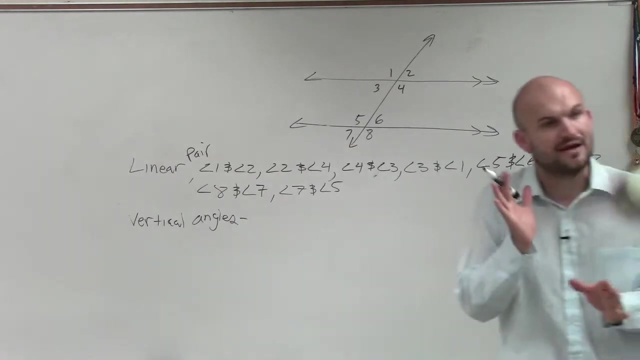 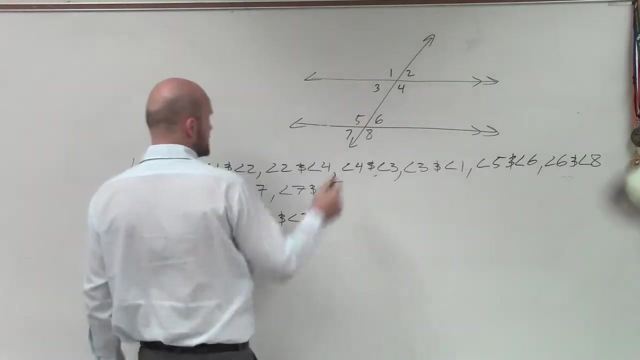 find all examples of yes. so the next thing is: you need to go over for vertical angles. so what are all the vertical angles? remember, vertical angles happen when we have angles that are direct, that intersect each other. so over here I could say angle 1 and angle 2, notice arm sorry. angle 4, sorry, do you? 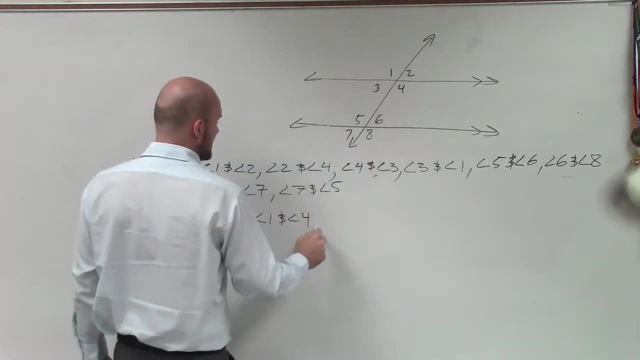 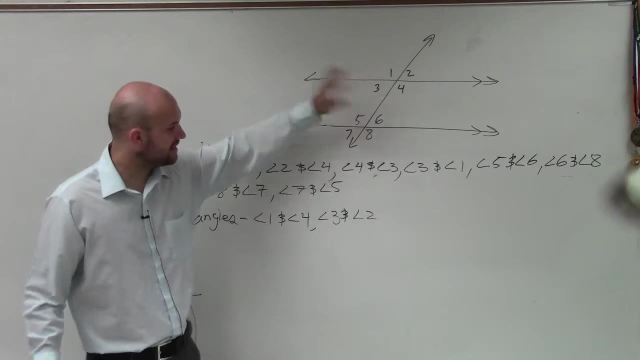 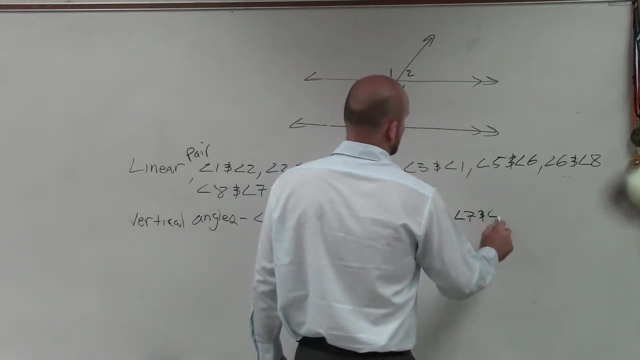 guys see how those are directly across from each other, off the intersection of these two lines. and also you have angle 3 and angle 2 over here you can say 5 and 8 and 6 and 7, angle 5 and angle 8, angle 7 and angle 6, all right, so those 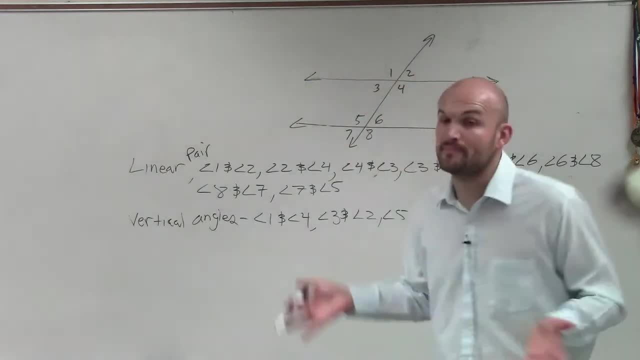 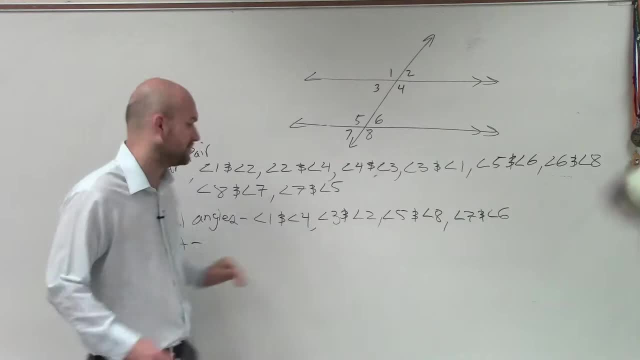 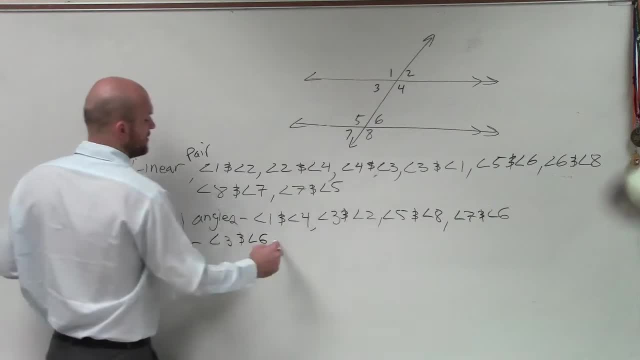 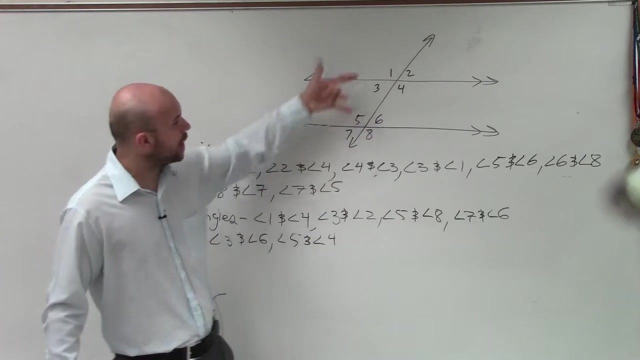 are angle 3 and angle 6, and then angle 5 and angle 4.. And there's only two examples of alternate interior. Then let's go to alternate exterior. So alternate exterior, ladies and gentlemen, are two angles that again are outside. now 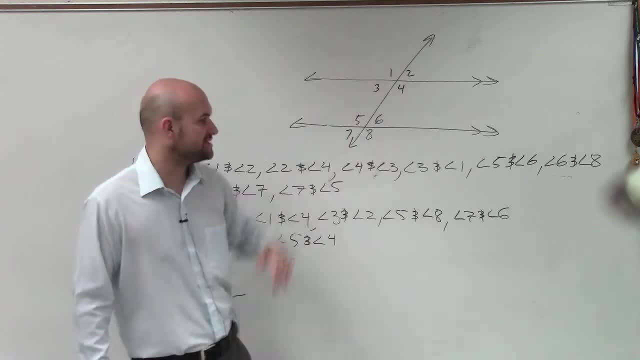 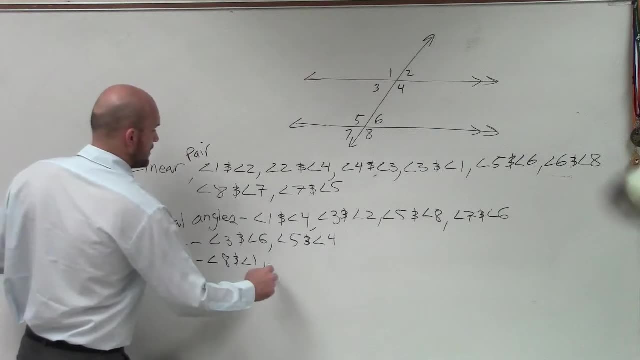 They're exterior of the parallel lines, but they alternate the transversal. So there, for example, those would be angle 8 and angle 1, and then angle 7 and angle 2.. So there's only two examples, Jessica. 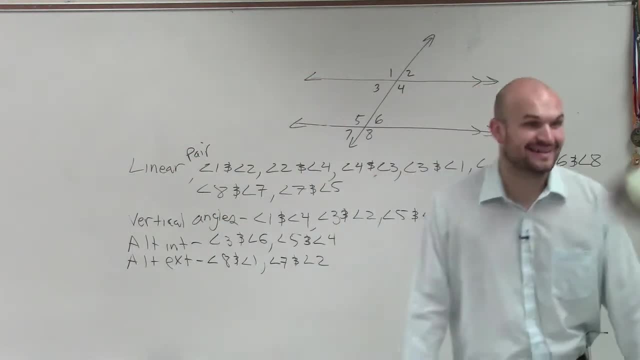 What are you talking about? There's not so many, I know, for a linear pair there's a lot, right, I know it's kind of crazy, But it's really important for you guys to be able to see SAM. 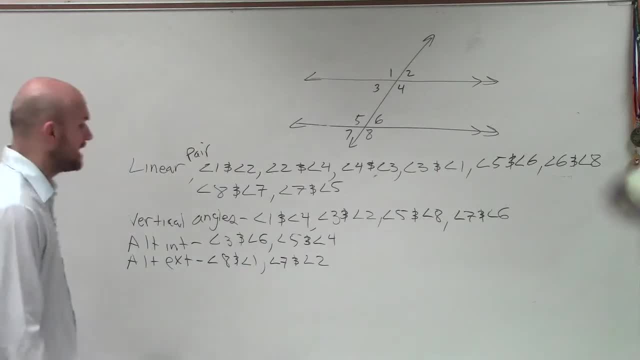 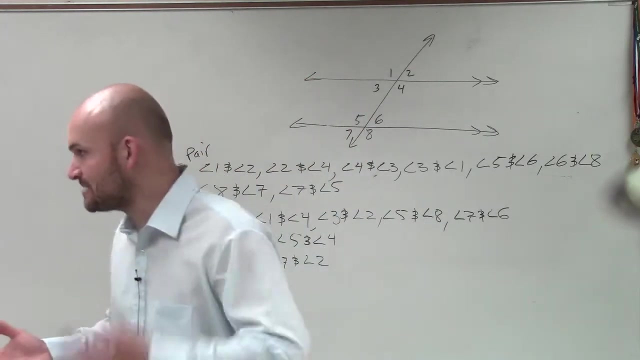 especially when you miss a class, to remember all of those and to have them written down as examples. The next one is consecutive Consecutive interior. Now remember guys: consecutive interior, consecutive, Think right next to each other, right, If you win consecutive basketball championships. 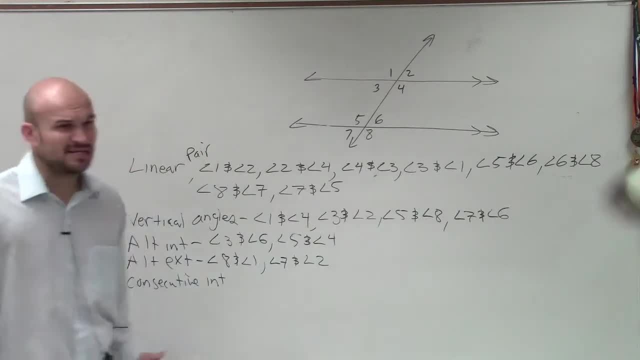 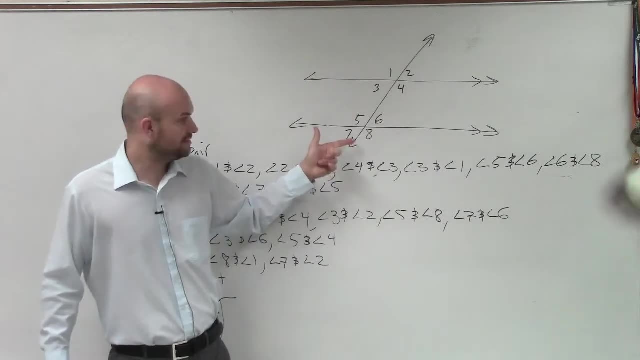 that's the one year, then the next year. A lot of people say: is it possible I have consecutive exterior? Well, if that's exterior and that's exterior, they're not consecutive right, They're not right next to each other.